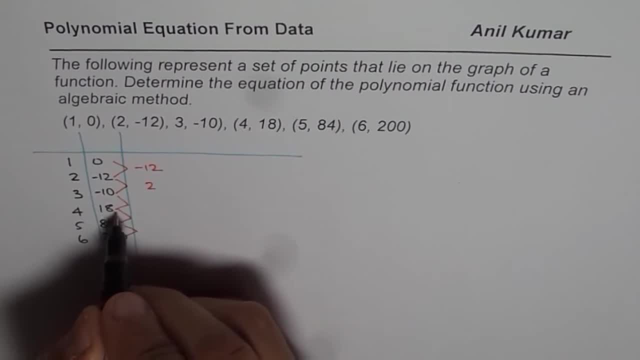 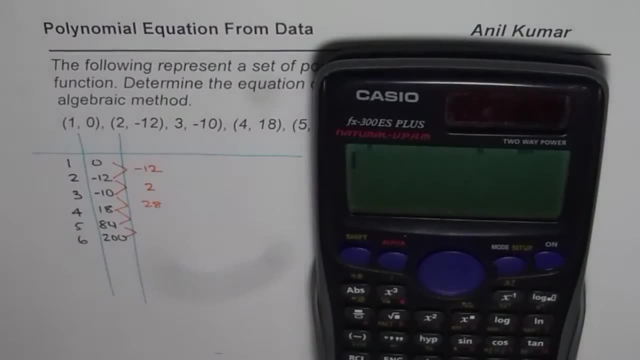 here Minus 10, minus 12 will be 2.. 18 minus this will be 28.. And 84 minus 18, we can actually use calculator. So we'll do: 84 minus 18 equals to 66.. 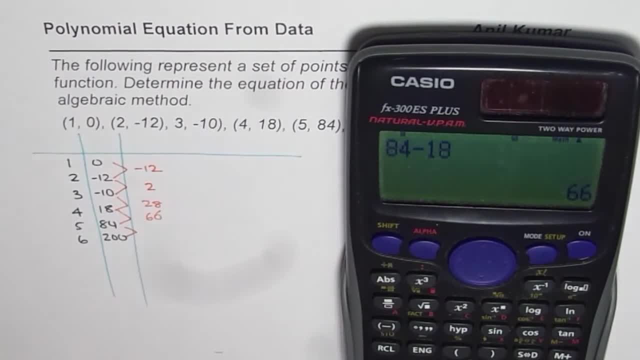 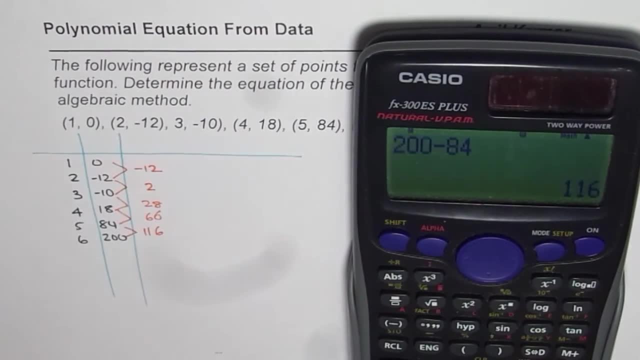 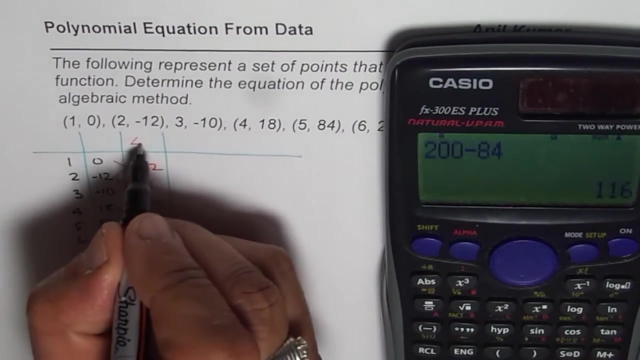 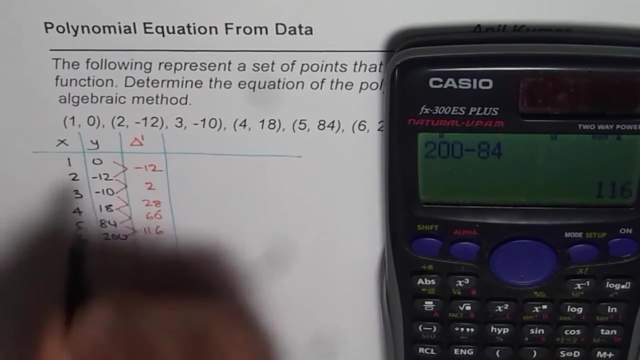 And 66, yeah, And 200 minus 84 is equals to 116.. Correct, Let us do the second difference now. So what we saw was that the first difference which I'm writing, as this is not constant, right? So we earlier wrote values of x and y which are given to us. Second difference: 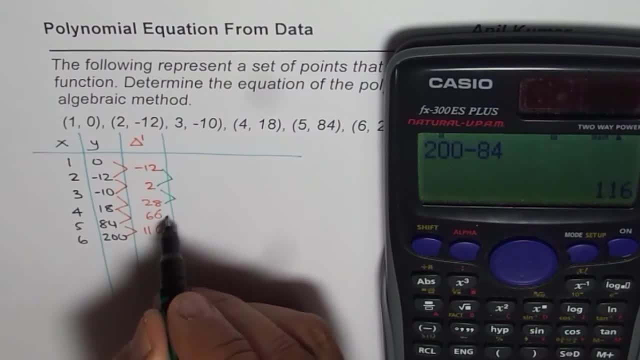 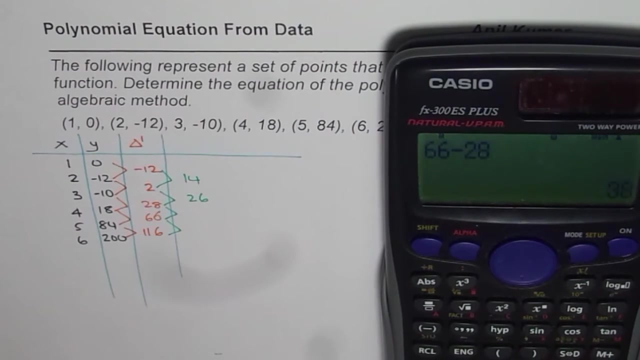 that is to do 2 minus 12.. So 28 minus 2, 66 minus 28,, 116 minus this, 2 minus 12 will be 14.. 28 minus 2 will be 26.. And then we'll show 66 minus 28, 38. And 116 minus 66 will be 50.. Now, that is also. 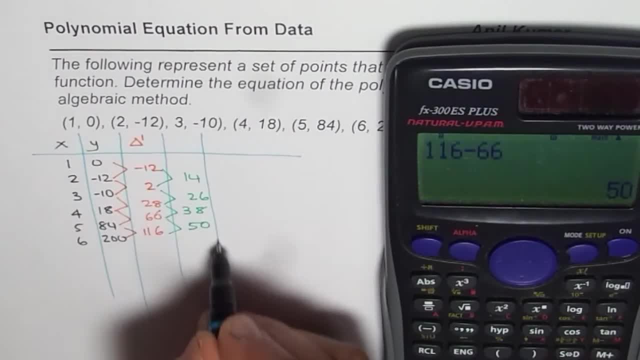 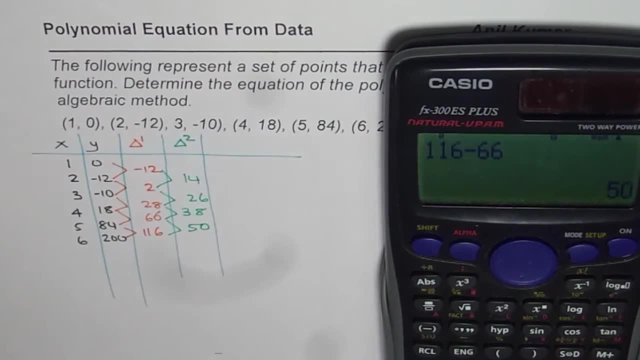 not constant. So we'll go for the third difference, right? So second difference is also not constant. So now let us find the third difference. So third difference: 26 minus 14 is 12.. 38 minus 26 is also 12. And 50 minus 38 is also. 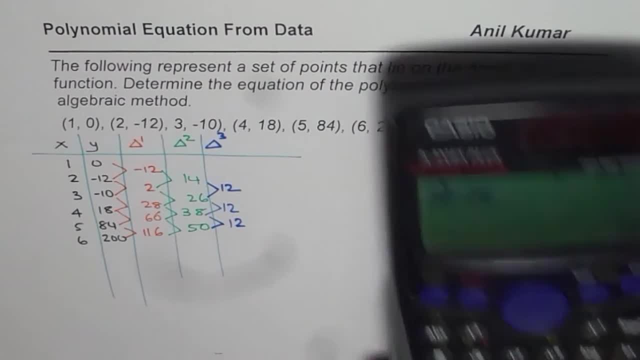 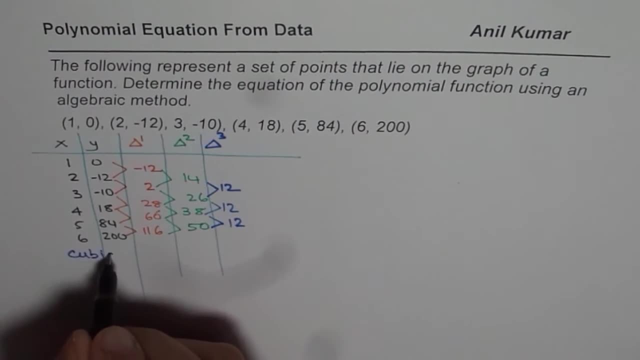 12. Now the third difference is constant for us. If third difference is constant, we know we are working with a cubic relation, right? So we have a cubic function And the third difference- delta 3, is 12.. Now if third, 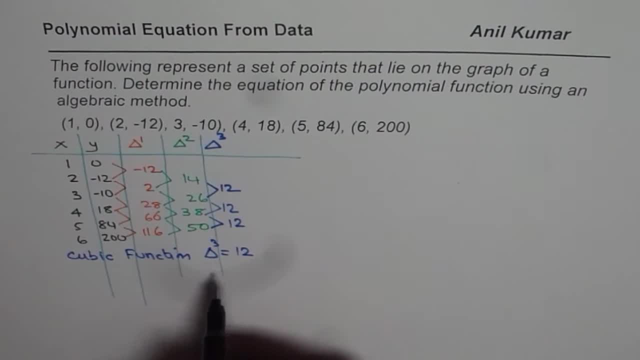 difference is constant. we can find the leading coefficient: A: A. the leading coefficient will be third difference, constant. third difference divided by 3 factorial. Now, third difference is 12.. 3 factorial is 12.. 3 factorial is 12.. So that's the third difference. Now let's 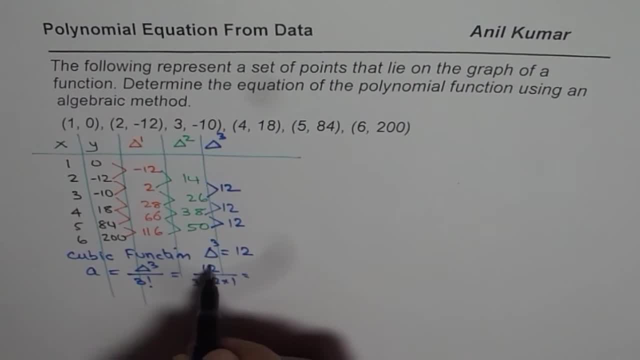 3 times 2 times 1, which is 6.. 12 divided by 6 is 2.. So the leading coefficient is 2 for us, and the equation of the function, which is a cubic function, a is 2.. So we'll write 2 x cube. 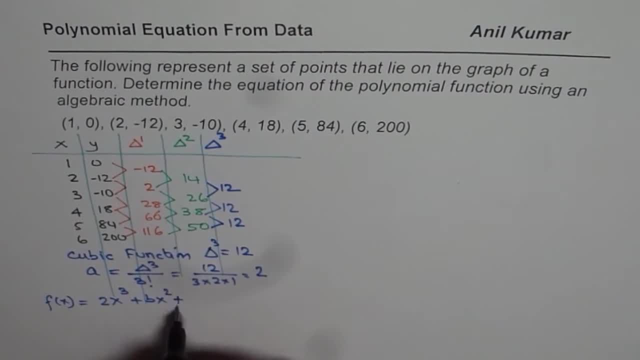 right plus bx, square plus cx plus d. So that becomes the equation for us. Now we are going to use these points to find the value of b, c and d. We have already found the value of a as 2, which I have substituted directly here. So that is the strategy. So we are trying to save some. 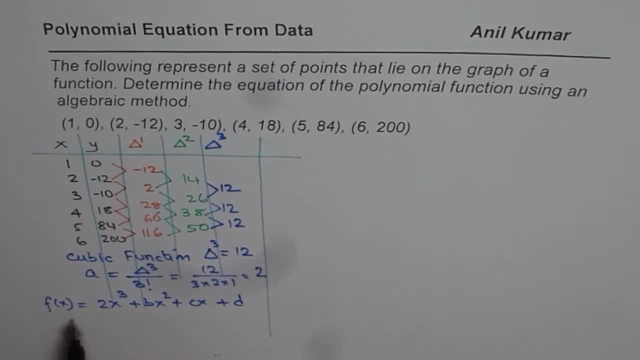 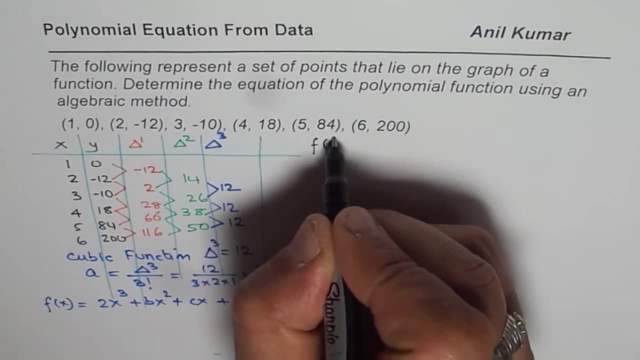 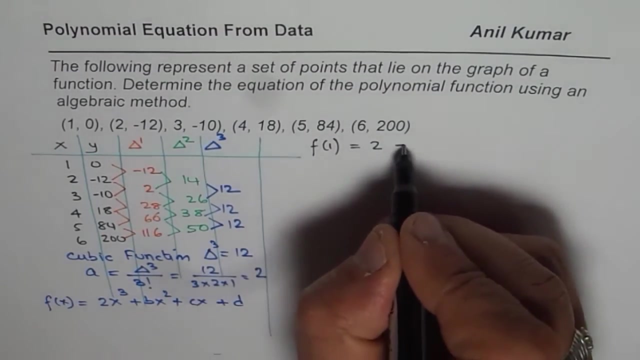 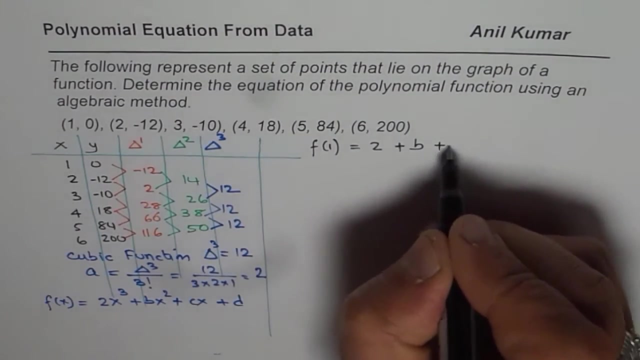 steps. Now, if I use the point 1, 0, that means we can write: f of 1 is 0.. So in this equation we substitute 1.. So we have 2.. 1 cube is 1. Plus b. right, We are substituting x equals to 1 and we have plus c. plus d equals to at 1, it is. 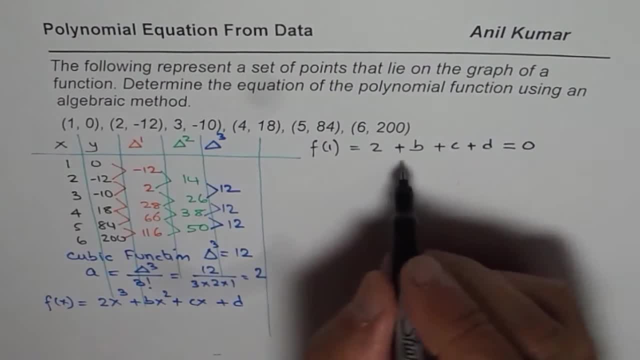 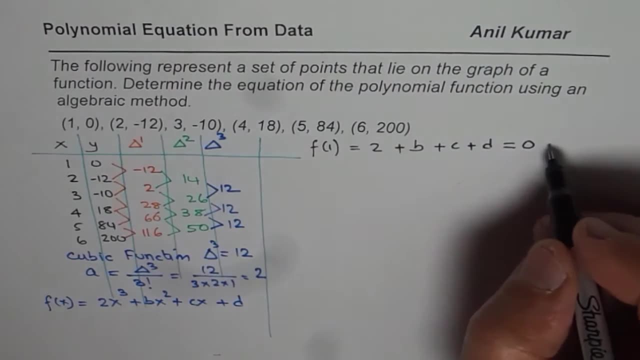 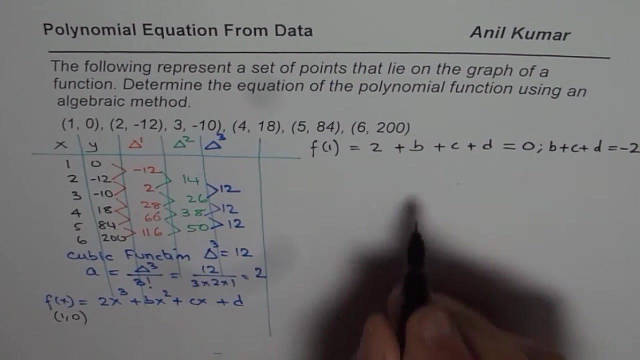 0. So this equation could be rearranged and we could write: b plus c plus d equals to minus 2.. So we can write this as. we can write this as, let me say, b plus c plus d equals to 0. So what we did was we substituted 1, 0. So we got the first equation. Now we'll substitute 2 minus. 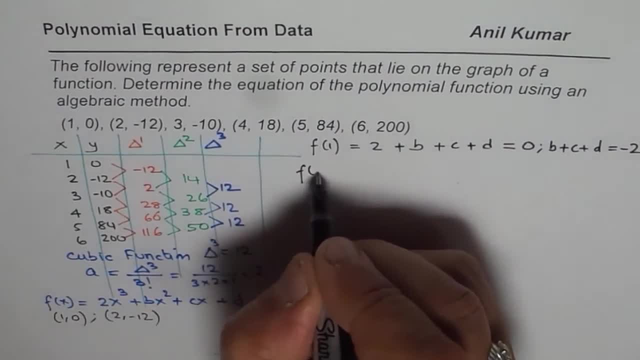 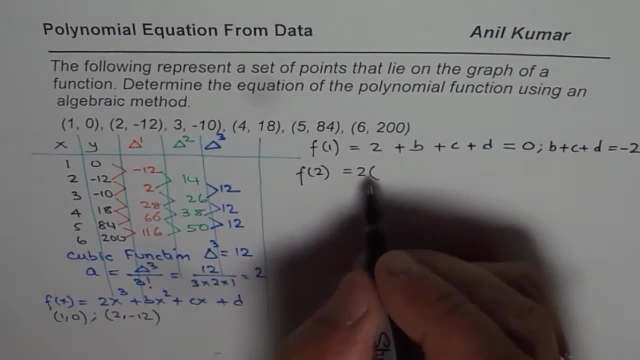 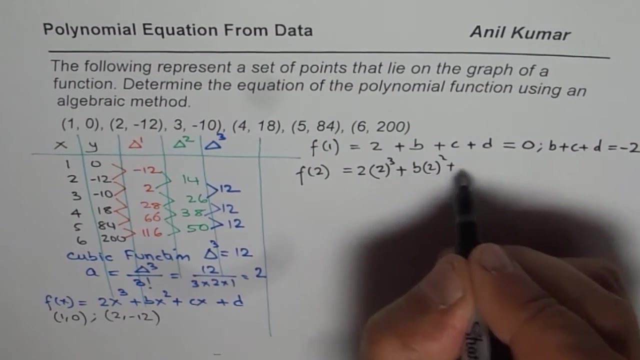 12 in the given equation. So we have: f of 2 equals to a is 2.. So 2 times 2 cube, 2 cube is 8.. Let me write 2 cube here first and we'll simplify this: b times 2 square plus c times, 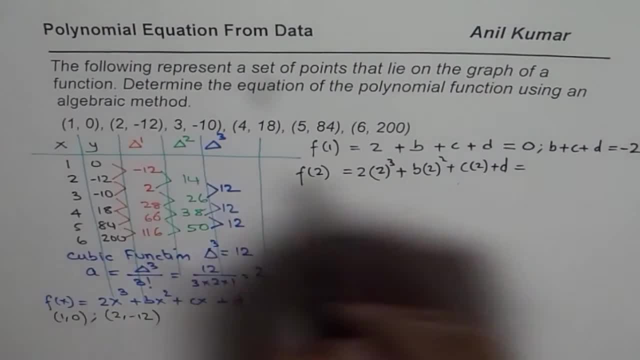 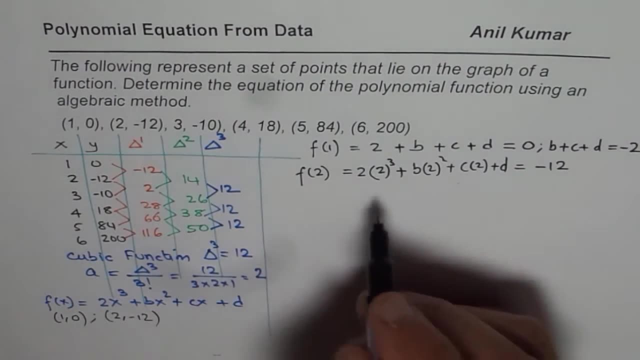 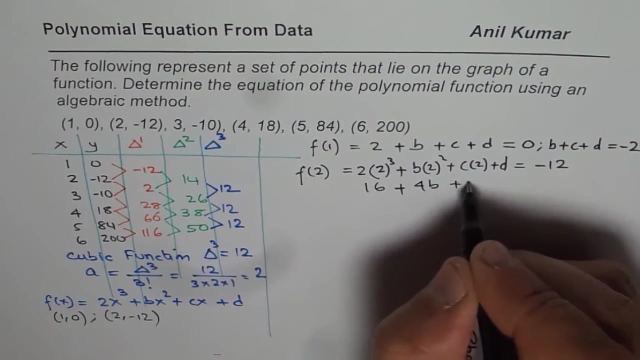 2 plus d, and this value f of 2 is minus 12, minus 12.. So let me rewrite this as: 2 cube is 8.. 8 times 2 is 16.. So we get 16 plus 2. square is 4.. So we get 4 b plus 2. c plus d equals to minus 12.. And 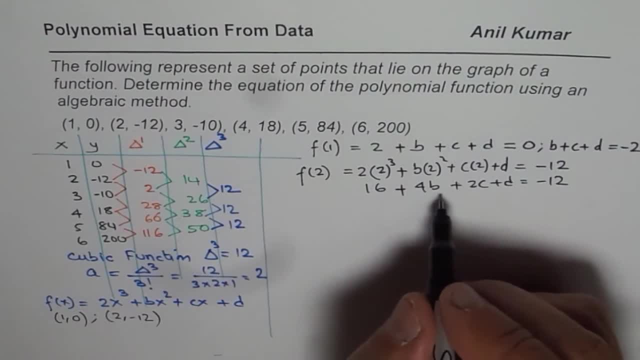 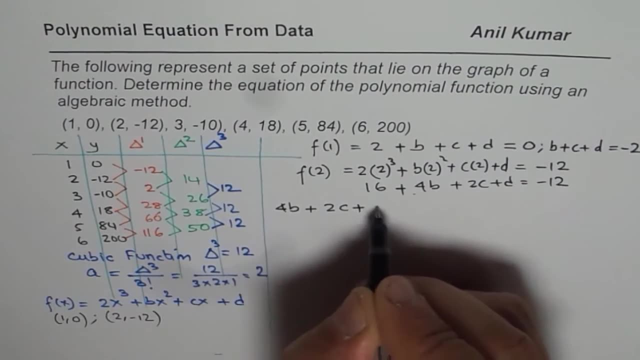 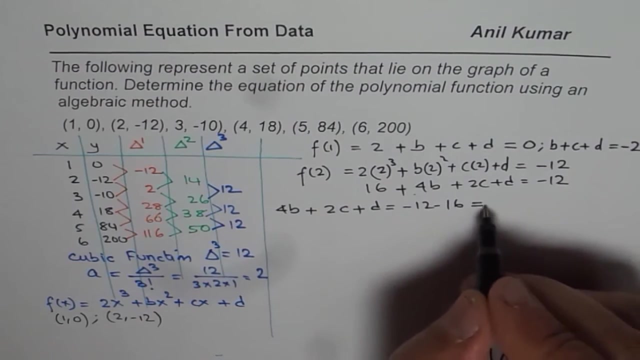 rearranging, we could write this equation as 4 b plus 2 c. So we could write this as 4 b plus 2 c. 4b plus 2c plus d equals to minus 12, minus 16, and that is equals to minus 28.. So that 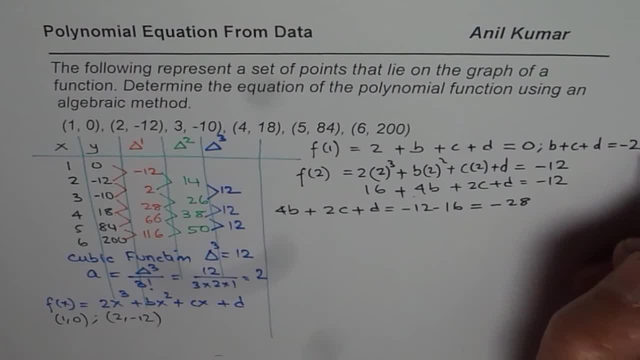 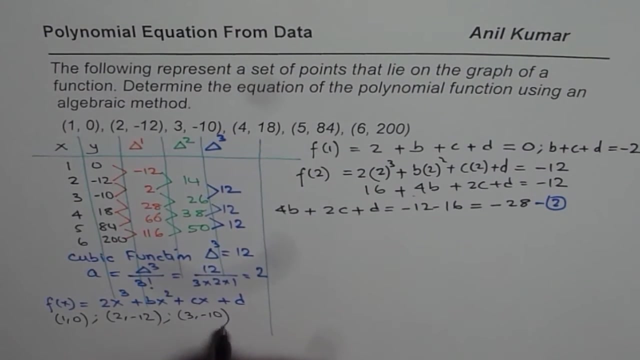 is the second equation. So what we will do here is we will write of these equations 1 and equation 2.. Since we need to find 3 variables, we will have to use 3 points. Third point is 3 and minus 10, 3 and minus 10.. Let's use that point also. So f of 3 will mean that 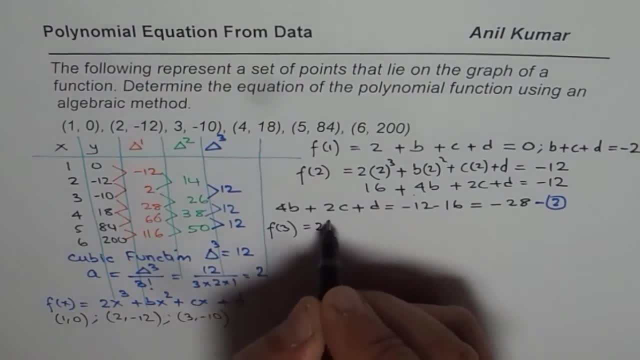 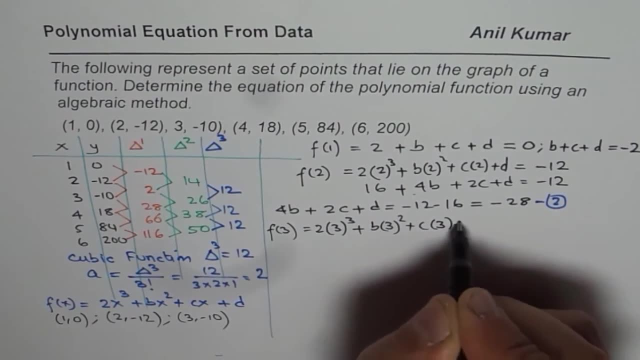 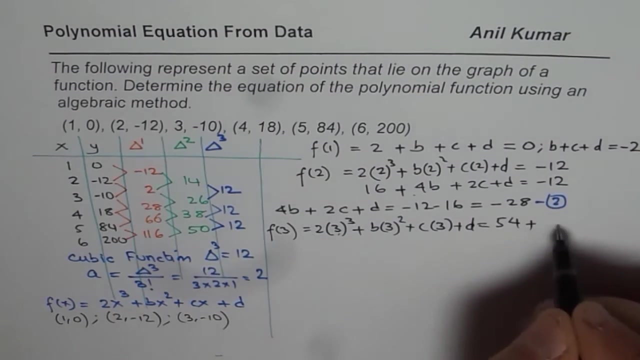 we have to write 3 here for x, So that is 2 times 3q plus b times 3 square plus c times 3 plus d, and that is 3q is 27,. 27 times 2 is 54 plus 3 square is 9, 9b plus 3c plus d. 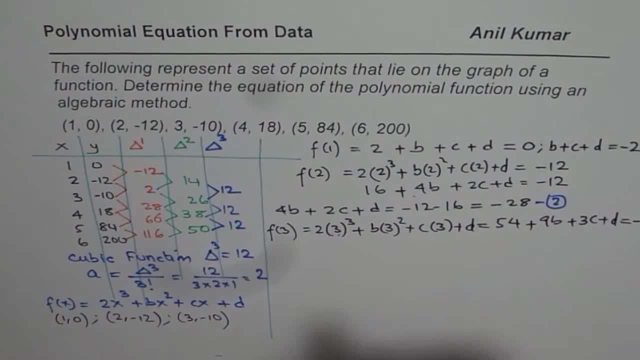 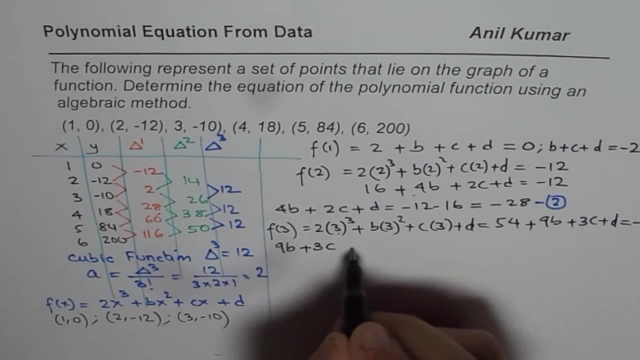 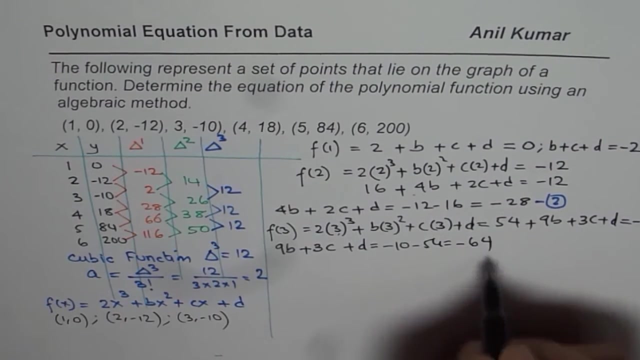 and that is Now we can rearrange this equation, also Taking 54 to the right side. so we get our equation as: 9b plus 3c plus d equals to minus 10 minus 54, which is minus 64. So we will call this: 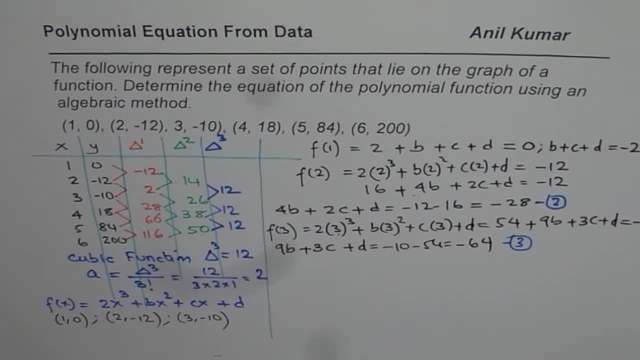 as our equation number 3.. Now, with three equations and three variables- these are simultaneous equations To solve, or what we can do is we have d as common. If I subtractif, I subtract one from the other, then we can find the value of find two equations in b and c. So what we will. 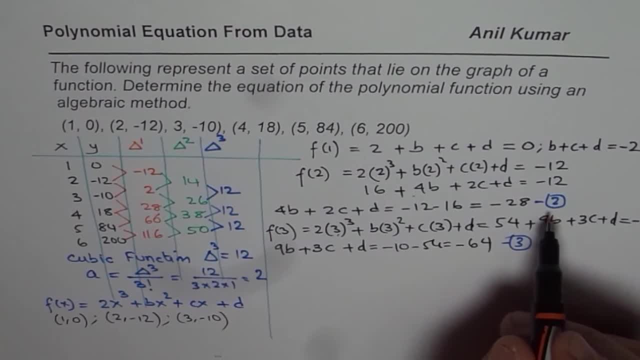 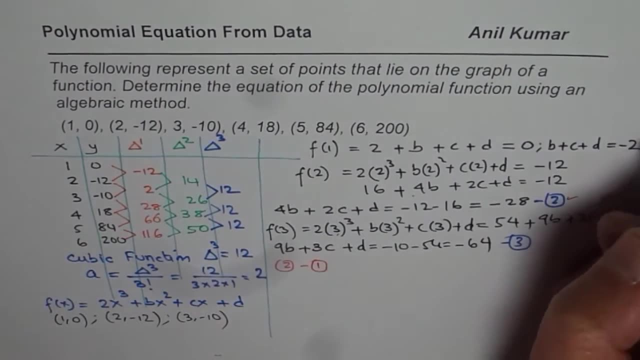 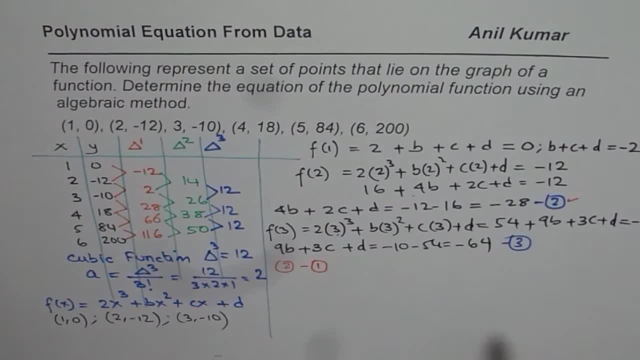 2, we have 4b. 4b minus b is 3b. So let me write this as 4b minus b is 3b, 2c minus c is c, So plus c, d, d. cancel out. So we have minus 28 minus 2.. So that becomes plus, That is minus 26.. 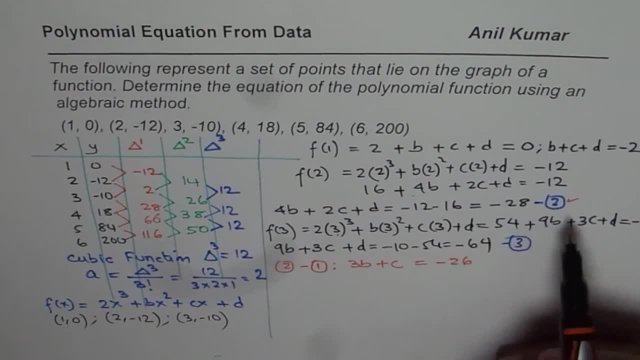 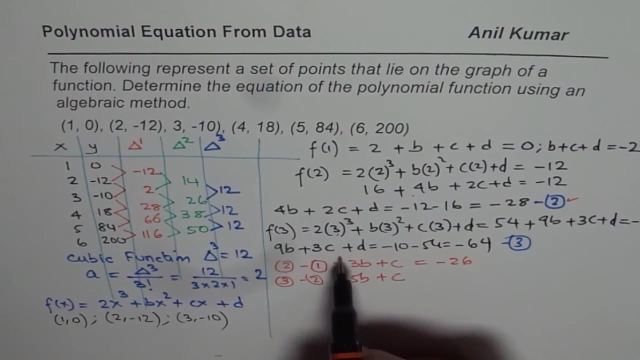 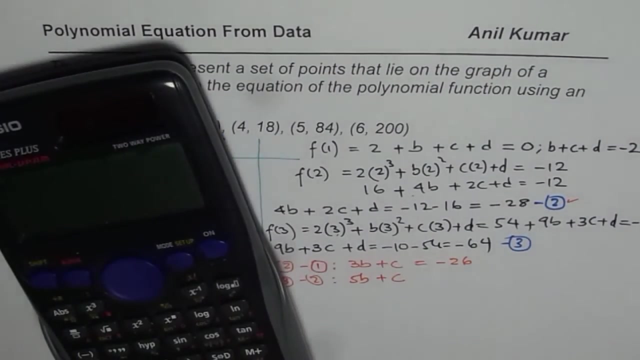 And now we will do equation 3 minus 2.. Equation 3 is 9b and this is 4b. That gives us 5b. 3c minus 2c is plus c And d and d cancel out Minus 64.. So we'll do minus 64.. So we'll do. 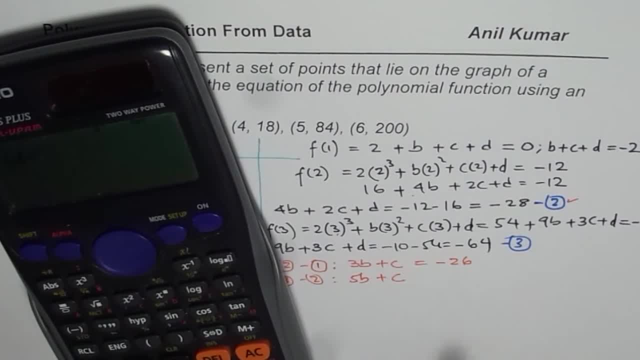 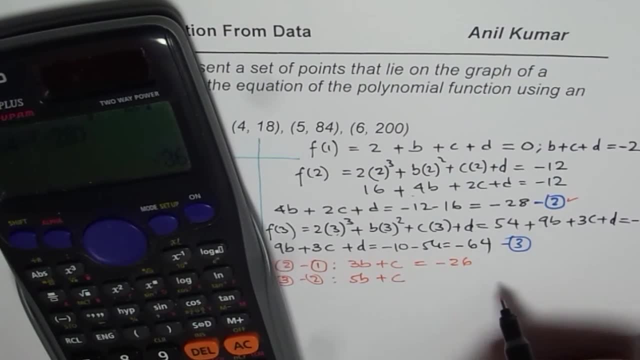 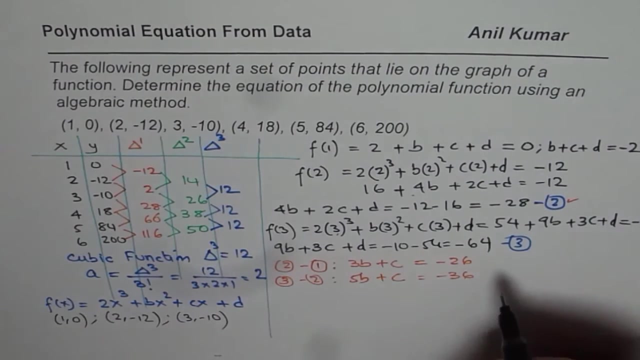 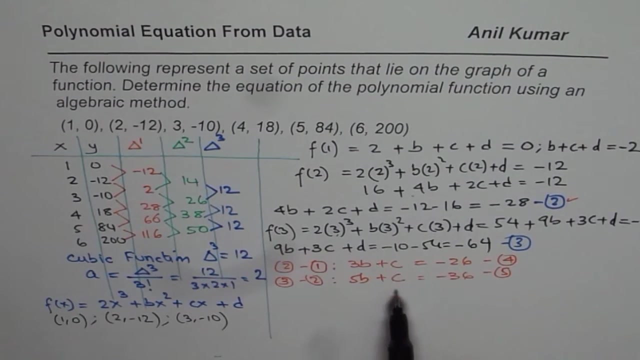 minus 64, minus minus 28.. So we'll do: minus 28 equals to minus 36.. So that is what we get. Let us call these equations as equation 4 and equation 5.. Now from these equations to eliminate c, we could: 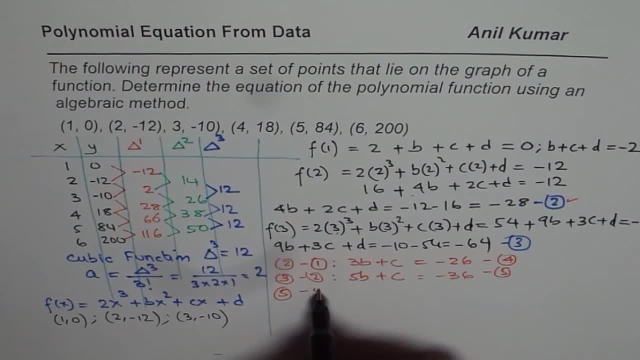 do 5 minus 4.. So we'll do equation 5 minus 4.. So when we do 5 minus 4, we're going to get our equation 2b, c and c cancel out equals to this minus, that is, minus 10, right So? 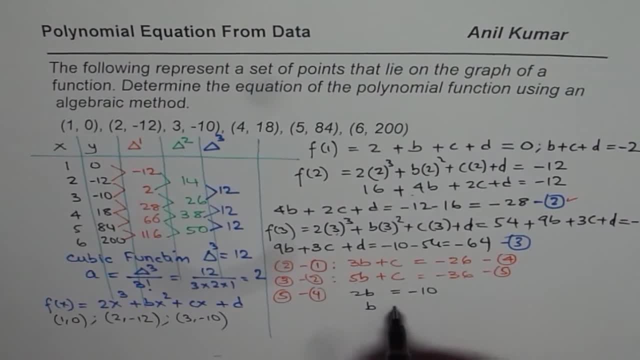 5 minus 4 minus 10.. And we can calculate b as minus 10 over 2 as minus 5.. So we get value of b as minus 5.. So let us call this as our equation 6.. Substituting b, we can: 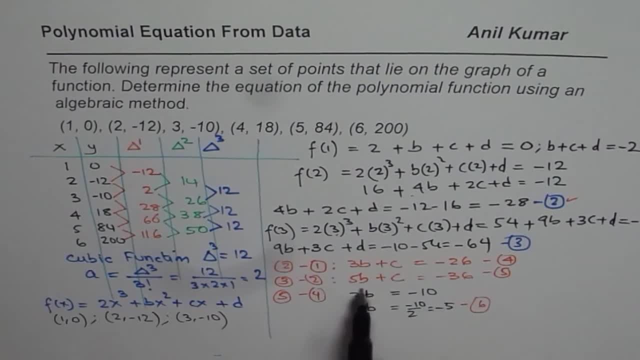 find c right. So if I substitute b as minus 4, we get our equation 2b, So we get our equation 2b. So if I substitute b as minus 5 in this equation, which is 5,, so we get 5 times b is minus 5. 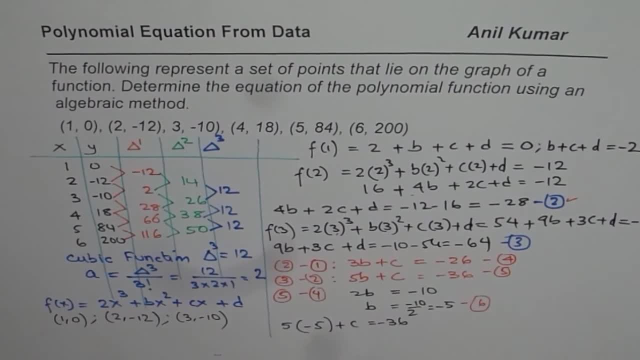 plus c equals to minus 36.. And from here we can say c is equals to minus 36.. 5 times 5 is 25 plus 25.. Is it okay? So when you do that, you get 11 minus right. So c is minus. 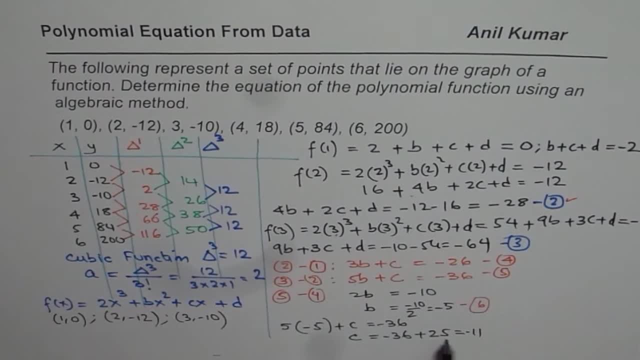 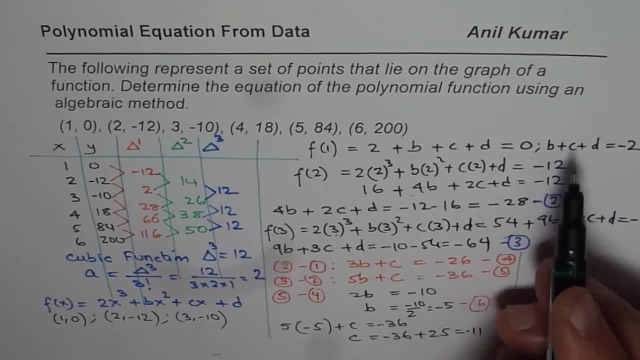 11 for you, 5 minus 36 plus 25.. So we know c now. So let us now find d using one of our original equations. Let me call this as equation 7.. And we will now substitute 7 in equation 1. 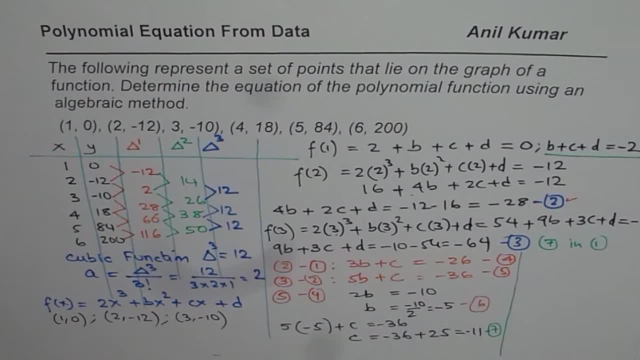 here right, And then try to find the value of d, b plus c. plus d equals to minus 2.. b is minus 5.. So we have minus 5 plus c is minus 11.. Plus d equals to minus 2. So we can find d from here. d equals to minus 2. And minus. 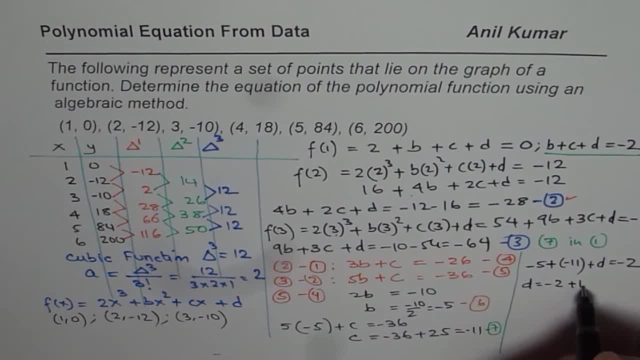 5 minus 11 is minus 16, which will be plus 16 on that side, So it is 14.. So we know d is 14.. So we get the value of d as 14, value of c as minus 11, value of b as minus 5.. Combining: 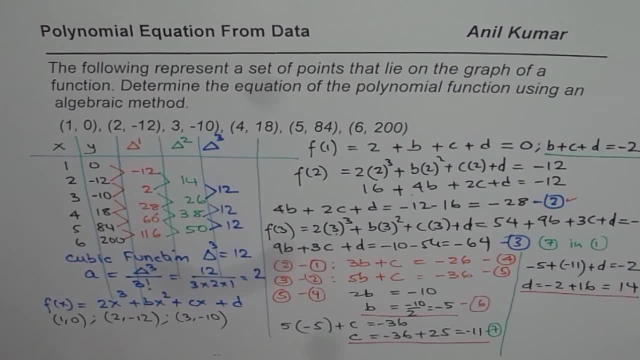 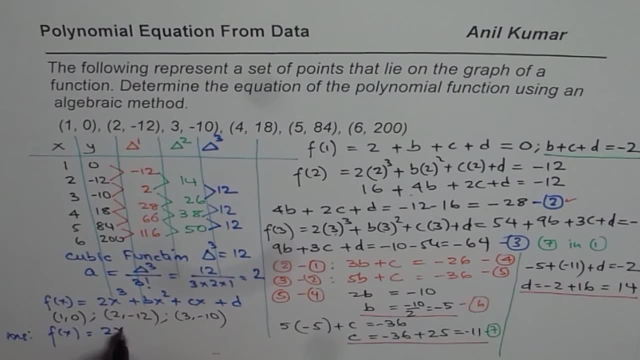 all these values, we can finally write down our function now. So our answer here is that function f of x is equal to 2x. cubed a was calculated directly from the constant third difference Plus b. b is for us minus 5.. So we can write this: 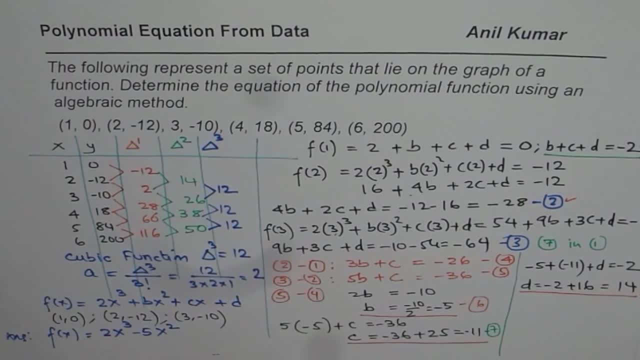 as minus 5x squared, c is minus 11, minus 11x plus d, which is 14,, so which is plus 14, right, So that becomes the equation for us. So that is the equation which represents the data for us. 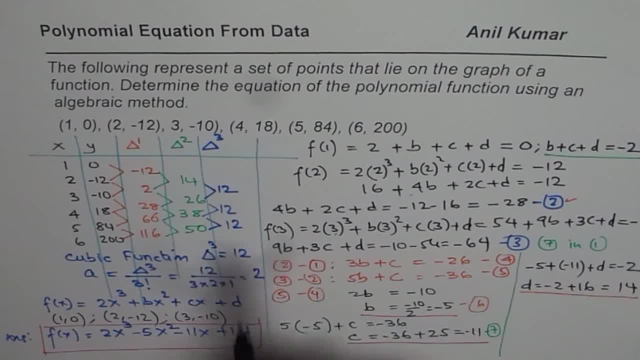 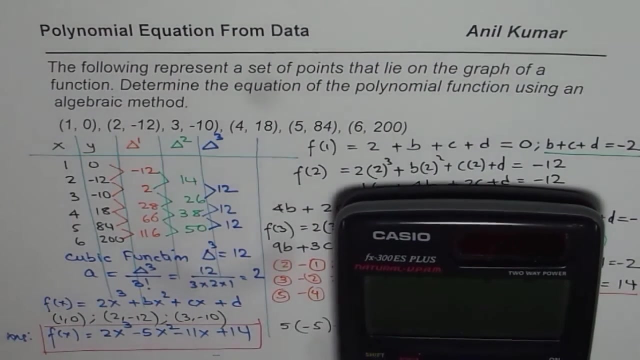 To check the result. what we can do is we can substitute a point and see: So if I substitute 4, what do we get? Do we get 18?? So that is what you could actually check. So let that be an exercise for you. Here is the check. So let us substitute 4 in our equation. So 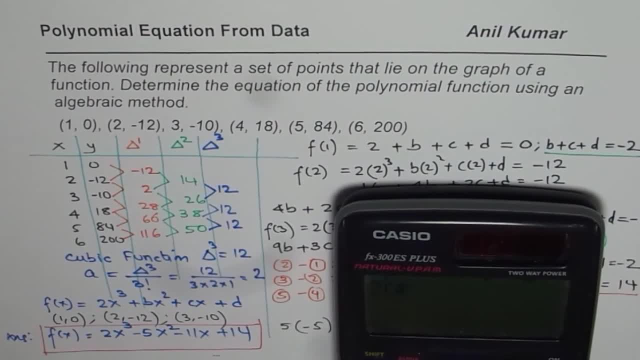 we get 2 times within bracket, 4 times 4.. 4 cubed minus 5x squared, so 5 times 5 times x is 4 for us. so 5 squared right Minus 11 times 4.. And then we will do plus 14.. And let us see, It is 18 for us, correct. 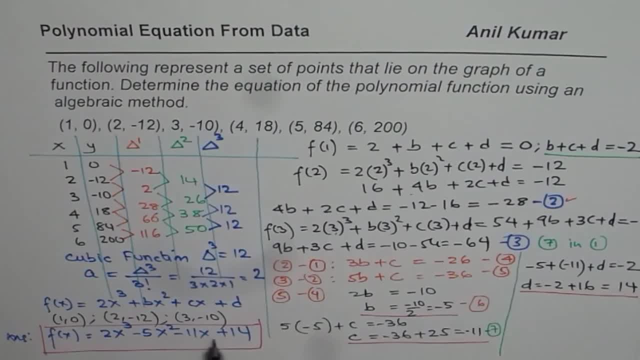 So it is 18.. So we can check our point also. So what we find is 6.153.. So if we find 7I, for example, there is a point right here. I will use that and I am that the point verifies that the equation is perfectly fine.